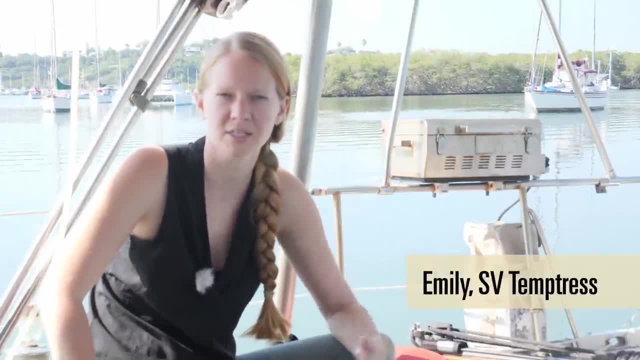 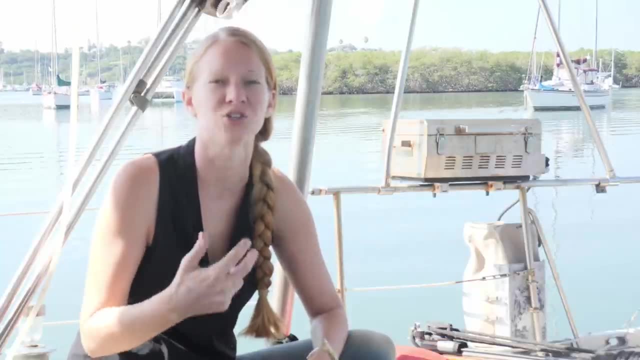 Hi, my name is Emily and I'm aboard sailing vessel Temptress. My husband and I sail and travel full time on our boat and today I want to tell you about knots, specifically the five knots that we use on our boat to get the job done, And I bet two of these knots are knots that you might. 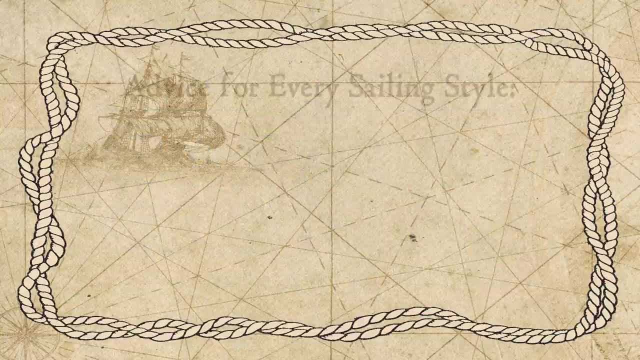 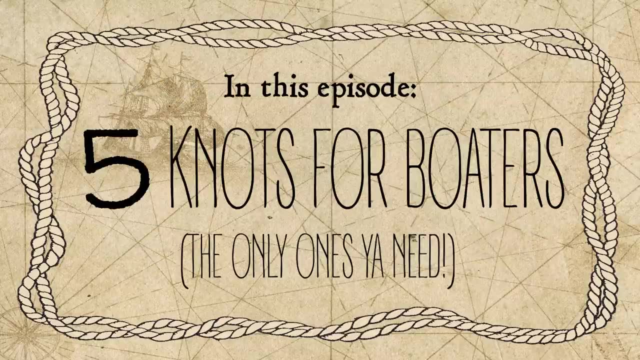 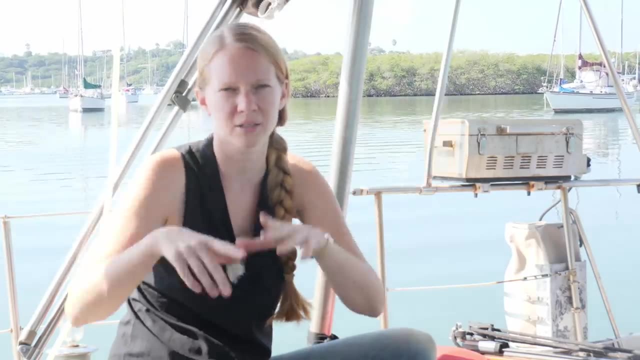 not have heard of before. So today we're talking about knots. If you've ever been to a nautical themed restaurant or bar, you've probably seen one of those plaques on a wall somewhere. It has 30 different knots on it with turks heads and all these fancy things, And people think that if 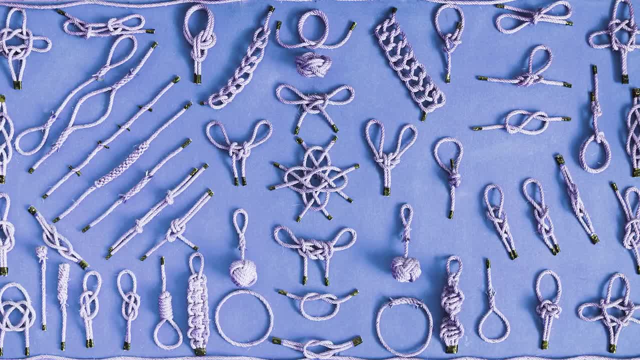 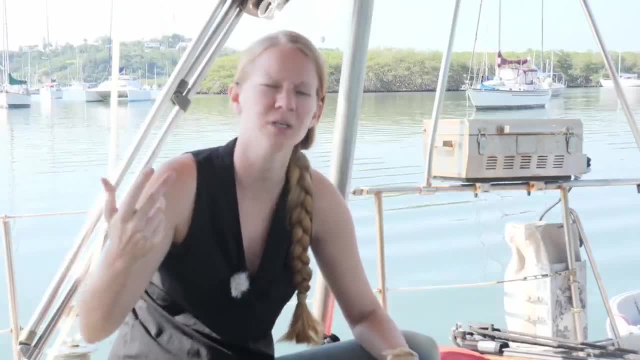 you're going to go sailing, you have to learn all these knots, but you really don't have to. The only knots you need are for basic jobs. You might want to put a loop in the end of a rope. You might want to put a loop in the middle of a rope. You might want to tie two pieces of rope together or keep. 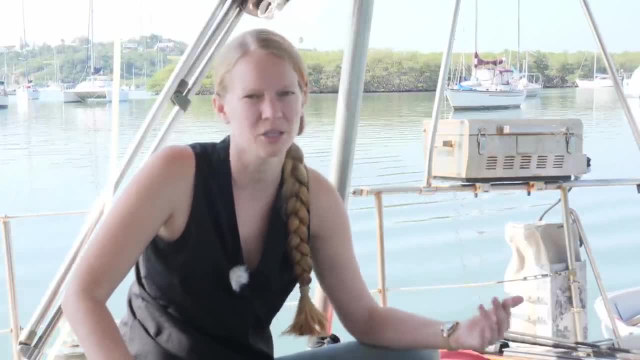 a rope from going through a hole that it's not supposed to. And lastly, you might want to tie something to something else. Maybe you're bringing your dinghy up to a dock or to somebody else's boat and you want to tie it to something else. And you might want to tie it to something else. 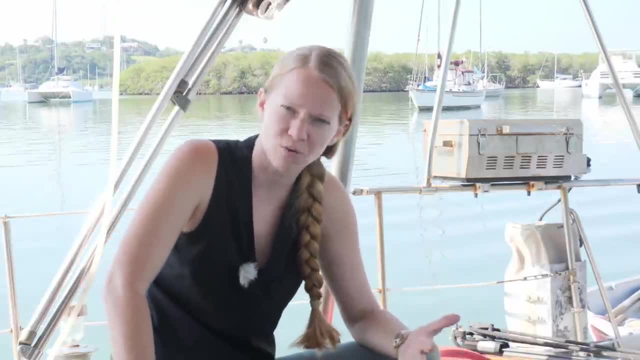 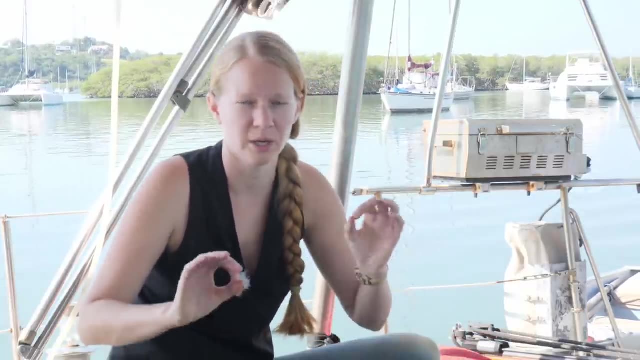 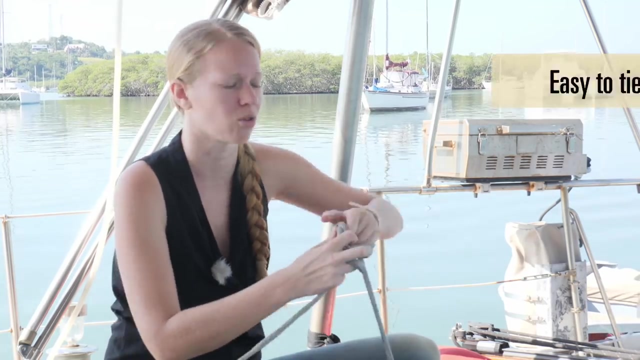 If you can do those five things, you're in pretty good shape as a sailor And the knots that we use are specifically great for those things. They're also great knots because the knots we use are knots that we don't have to think a whole lot about. We can kind of tie them without looking. 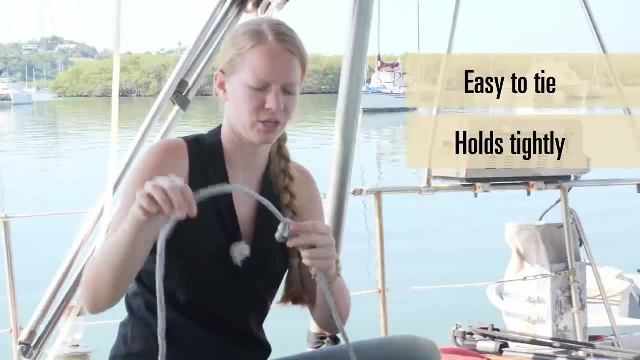 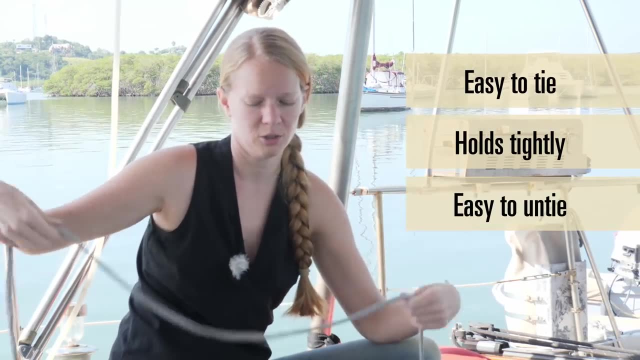 at them. They're also knots that hold well when you put them under pressure and they're easy to break apart, so that when you take the knot out you're left with an undamaged piece of line. So those are the great knots that we use. 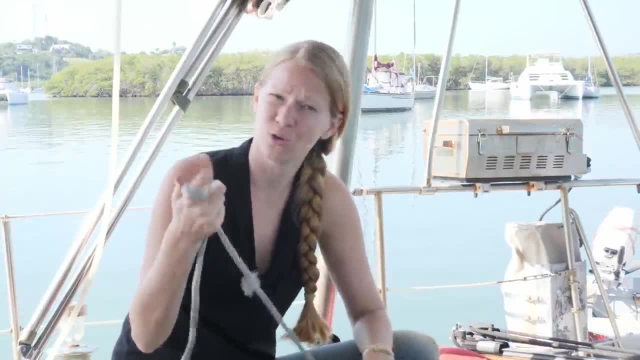 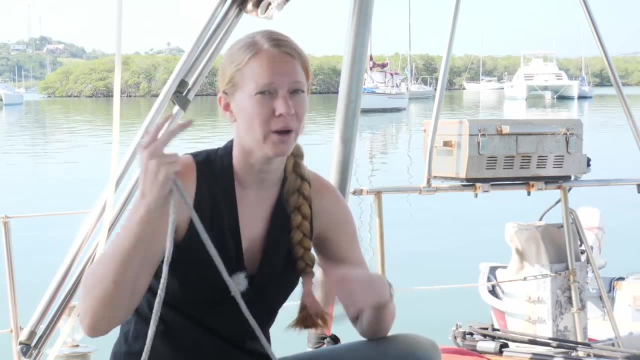 When you've mastered a knot, you will know it, because you will be able to know when to use it. You'll be able to tie it, and you'll be able to tie it under pressure when the boat is rocking or something is going wrong and you need to get it done right away. So I challenge you, as you're. 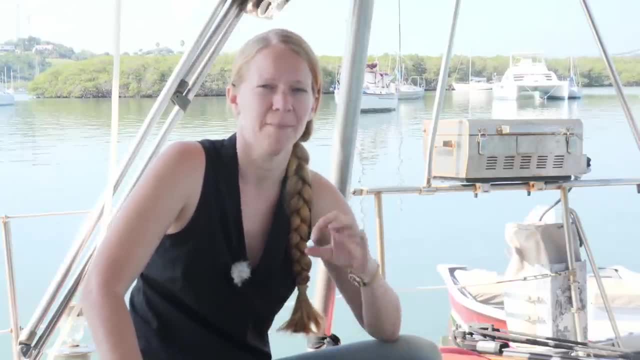 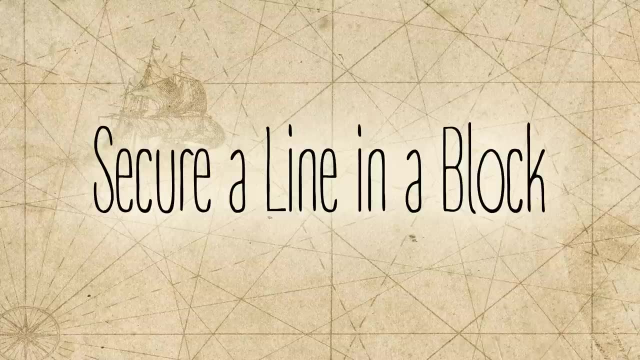 going through these five knots. you can pause the video. you can practice how to tie it. Make sure that you know how to tie them, and tie them quickly, and that you know what they're used for. All right, knot number one is a sailor's knot. 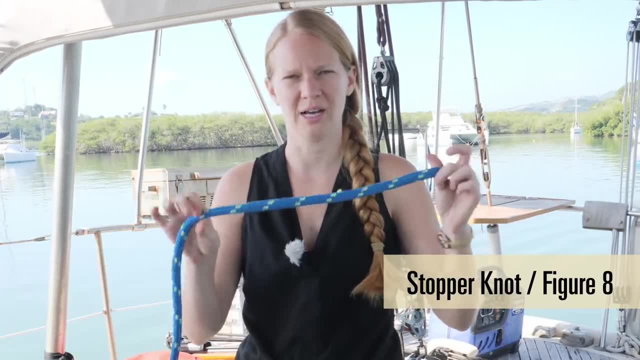 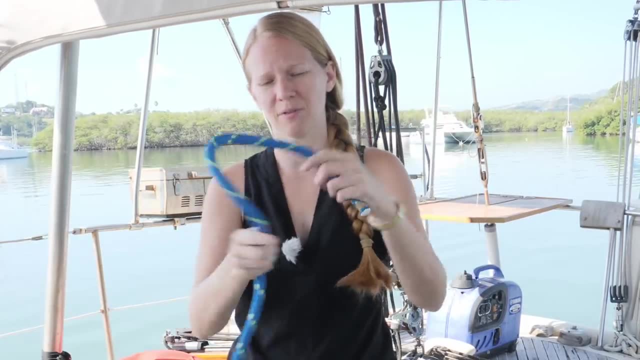 It's a stopper knot or a figure eight knot. When you're on a boat, if you've got a line and it's going through a block, you want to make sure it doesn't pull out of that block and go crazy. so you can't find it. So instinctively people usually want to tie an overhand knot- Pretty easy knot. 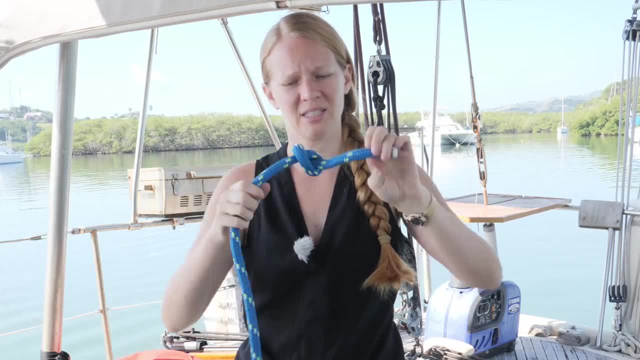 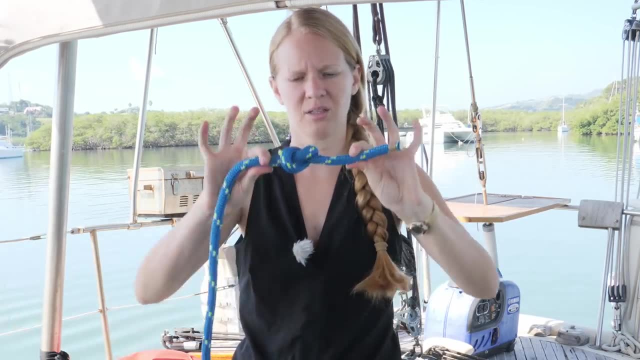 we're all familiar with it, right? The problem with an overhand knot is that the more tension you put on it, the tighter this knot gets, and sometimes it becomes nearly impossible to get that knot back out again. The other thing is this doesn't really add a ton of width to your line. 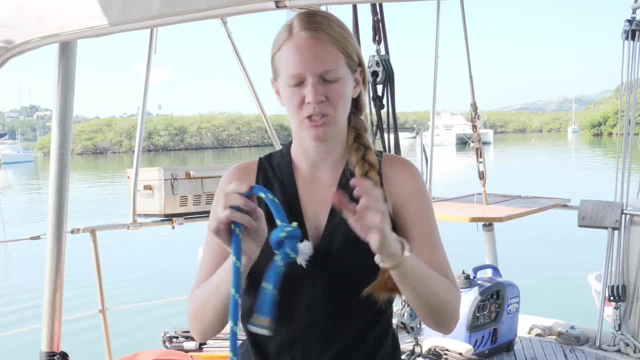 so sometimes you'll have to, you know, add a little more tension to it. So when you're on a boat and second one and it's just not a good knot to use. But there's a very easy variation to this that makes it the perfect knot to use. 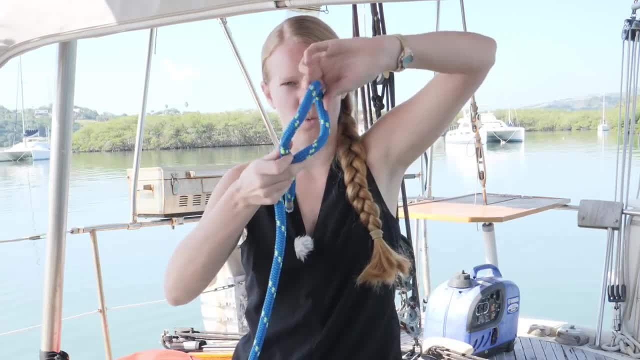 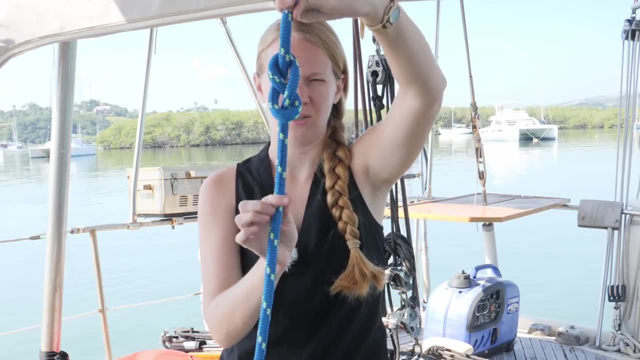 If you know how to tie an overhand knot, all you have to do is give it one extra twist before you put the end in and you have a figure eight knot. You can see it looks like a figure eight. that's why it's called a figure eight knot. 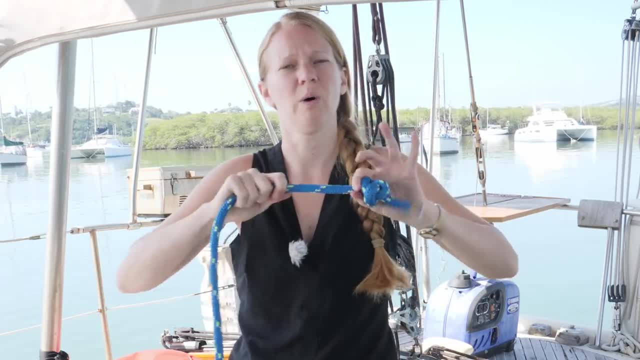 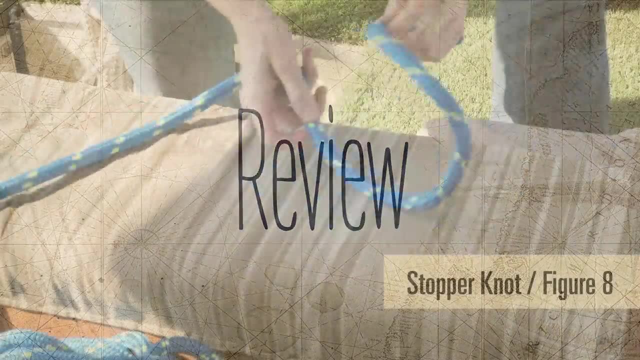 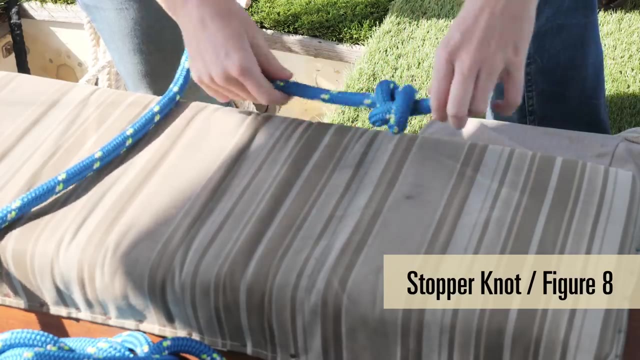 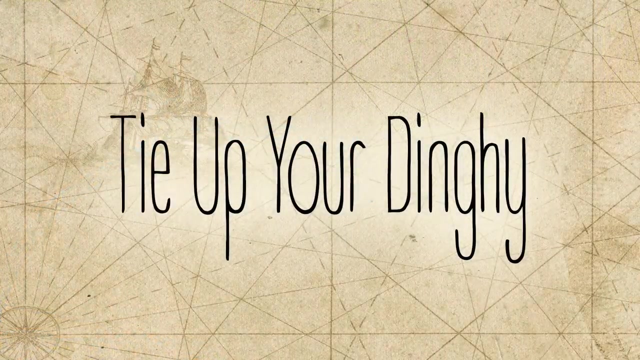 When you slip it down, it becomes bigger than an overhand knot and it works really well for keeping lines from going through blocks when they're not supposed to. Now let's talk about tying something to something else. This is going to come in handy when you're using your dinghy and going to a dock. 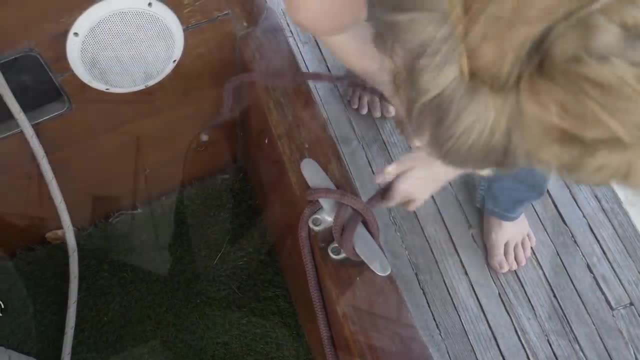 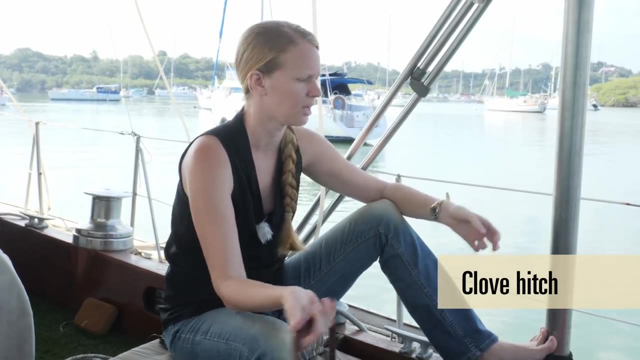 If there's a cleat there, you could just use a cleat hitch and tie off. but sometimes you don't and sometimes you have to tie off to something, Something we like to tie off to something, Something we like to use, for that is called a clove hitch and it's super easy to tie. 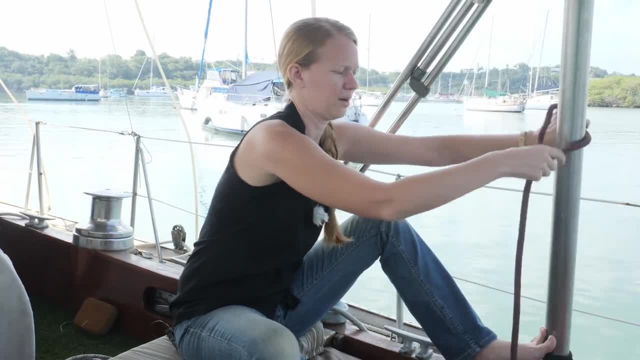 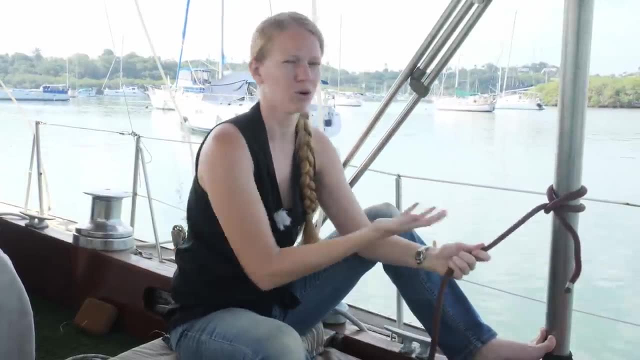 This is what a cowboy would use to tie his horse up. You put it around whatever you want to tie, to put it under, put it over, pull it through the loop And it looks like a knot. that's not very secure but it is secure. 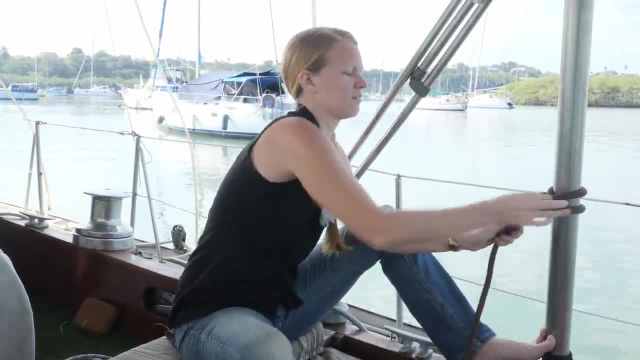 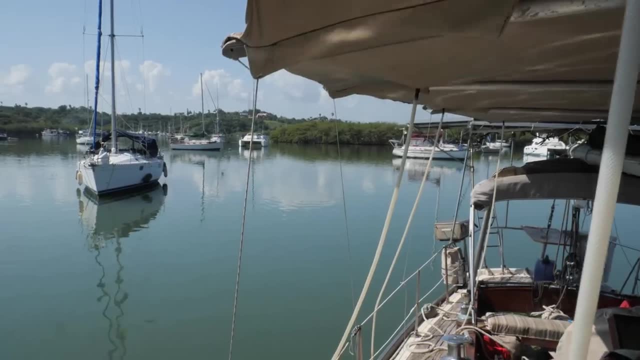 If you're really concerned about it, you can tie one more little hitch in the end of it to secure it and it looks a little more secure. but it's just fine the way it is. This is what we use to tie down our awning. 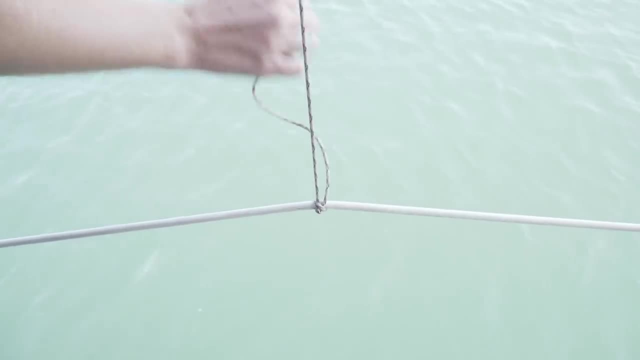 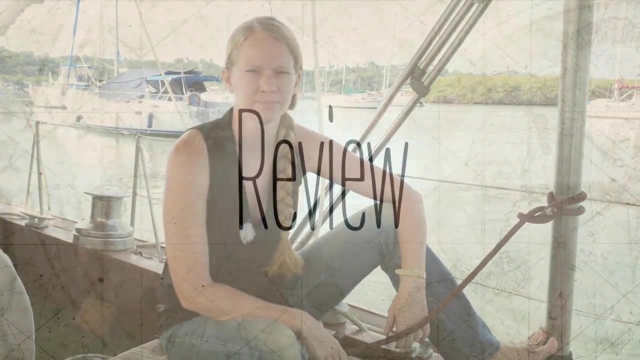 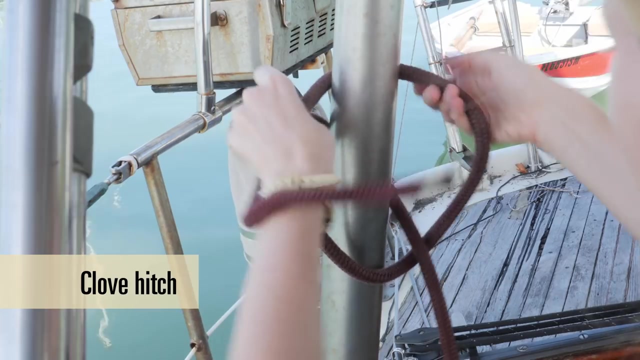 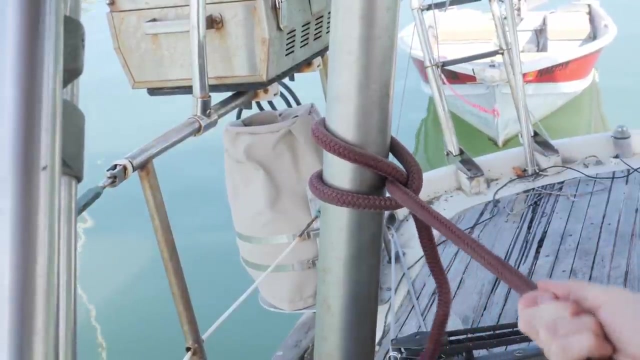 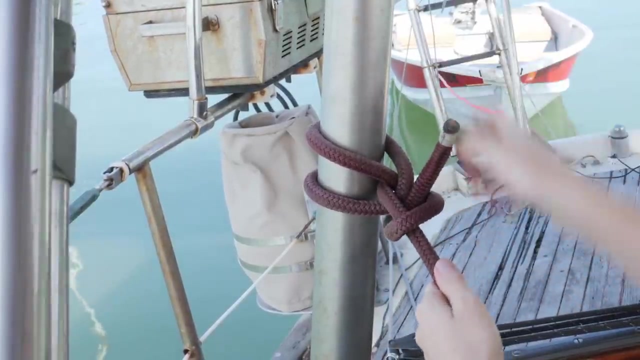 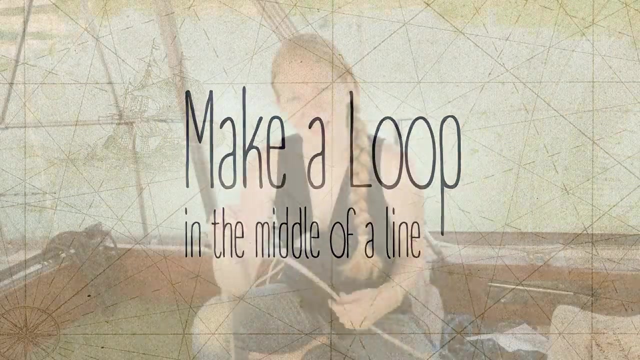 We leave a little loop in the end So it pulls right out and we don't take that awning down unless it's like blowing 30 knots. So it's quite a secure line. So that is a clove hitch. Next let's talk about putting a loop in the middle of a piece of line. 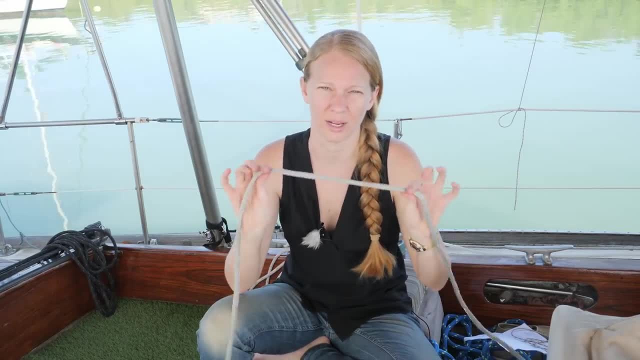 Now this line. I don't have access to the end, but that's not a problem, because we're going to tie it right in the middle with something called an alpine butterfly knot. This is a great knot, for if you go to the hardware store and you buy something, you 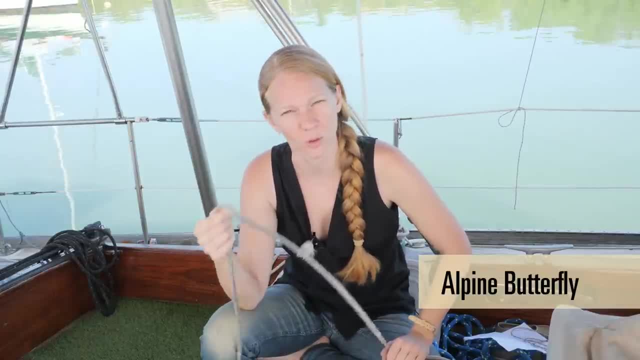 need to strap it down to the top of your car and all you have is twine. This is what we use to tie my dinghy down during crossings, So what you're going to do. if you've ever played Cat's Cradle, it's kind of like that. 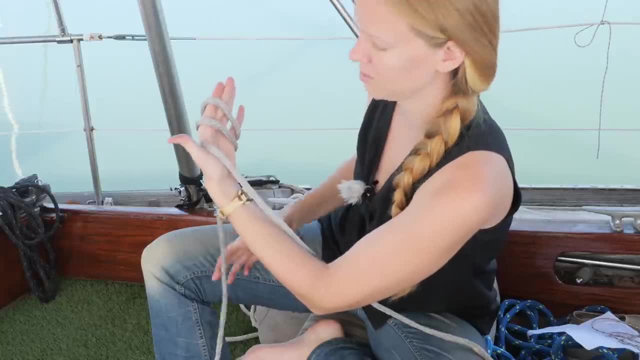 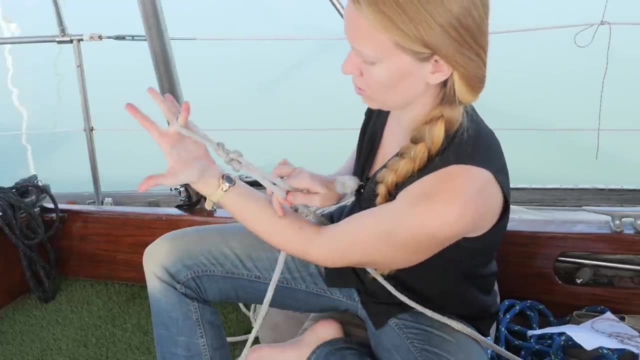 You're going to wrap the rope around your hand three times. you're going to reach under the first one, grab the second one, pass it to your middle finger and slide it all over. So the only thing you're holding onto is the middle finger. 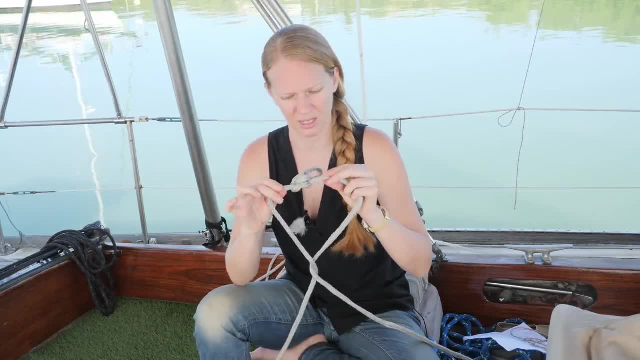 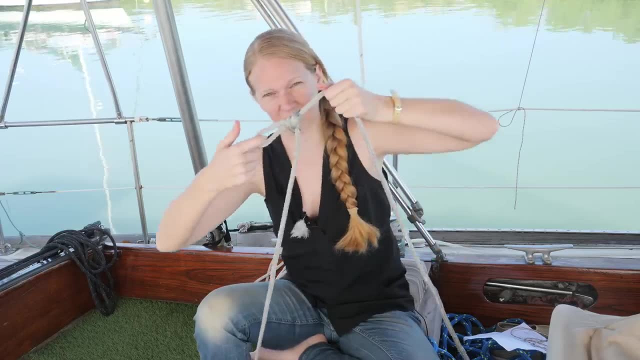 And then you pull There, you go And that is an alpine butterfly knot. This is. you can put another piece of line through this and use it as kind of a lever to give purchase and really pull something down tight, which is why we like to use it. 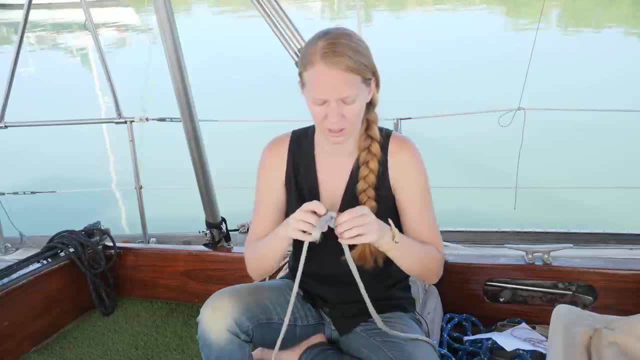 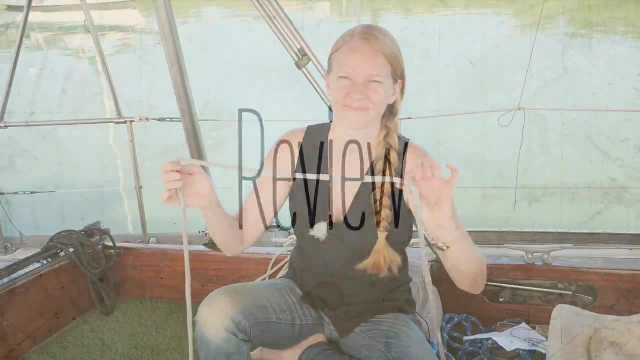 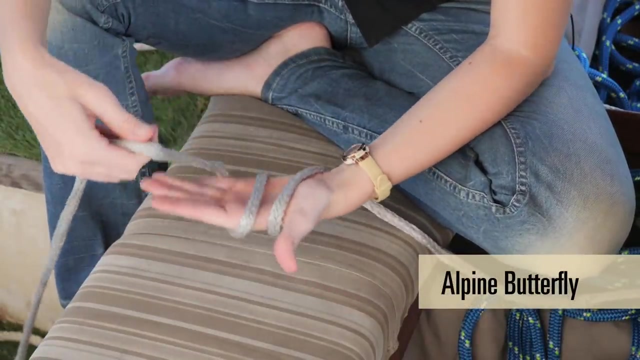 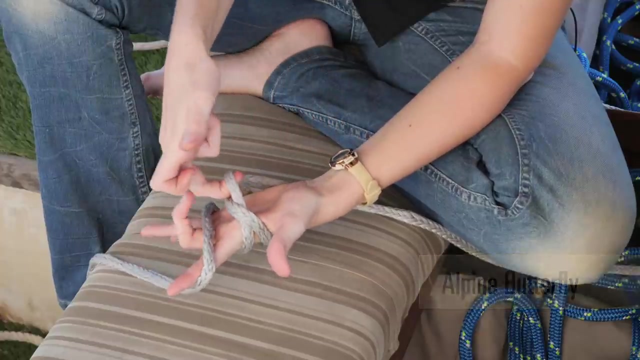 And of course it follows that rule: where there's these little backs you can break and get the knot right out back to nothing. So that is an alpine butterfly knot. And of course, if you're using a jib, where you're holding onto a piece of wire, you're 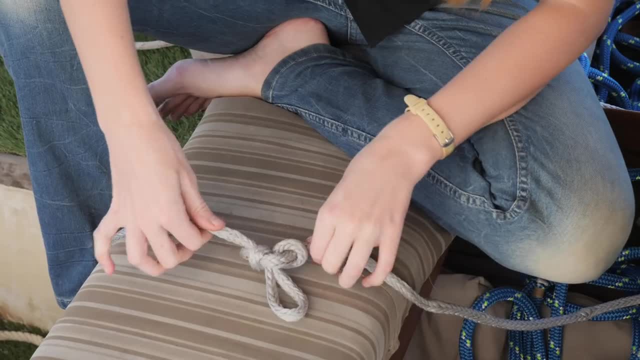 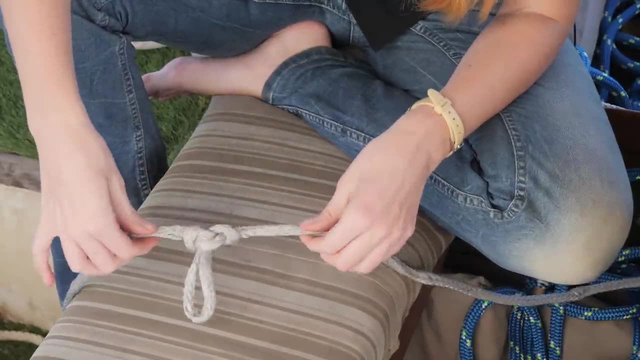 going to want to move the string just a tad bit back to the center of your knot to be able to pull it right out. So in this case, if you want to do a little bit more wiggle with your string, go ahead and do that. 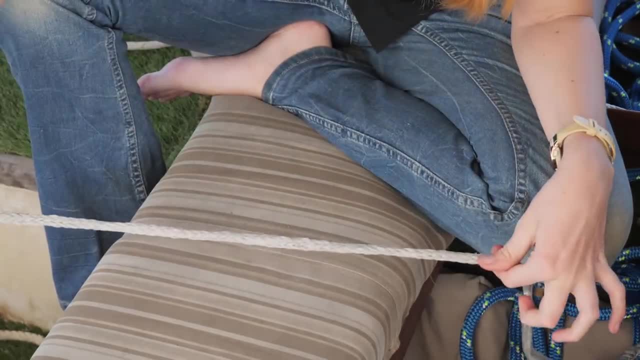 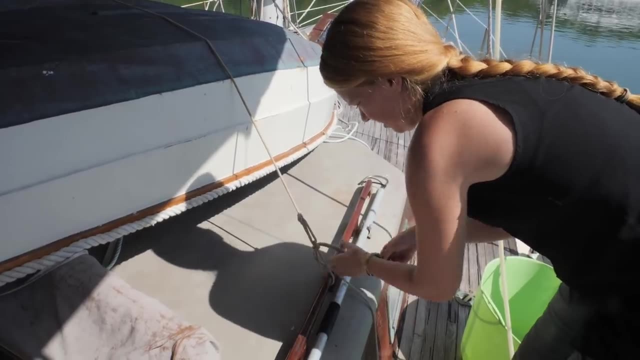 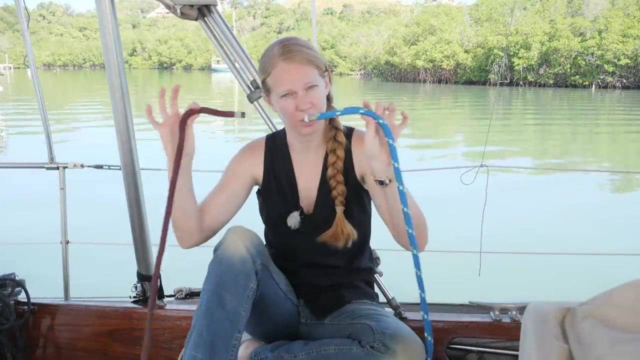 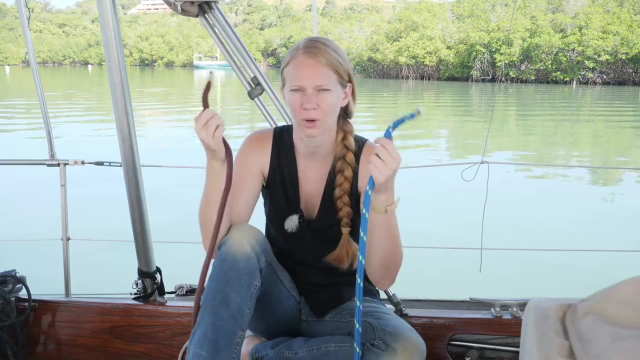 You're going to need a little bit of a knot. The first one to go. the next thing you might want to do is put two pieces of line together. sometimes you've got a 50 foot line and another 50 foot line and you really need 100 feet of line. so how do you put? 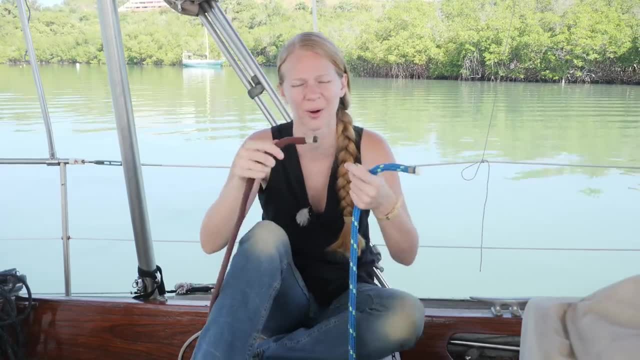 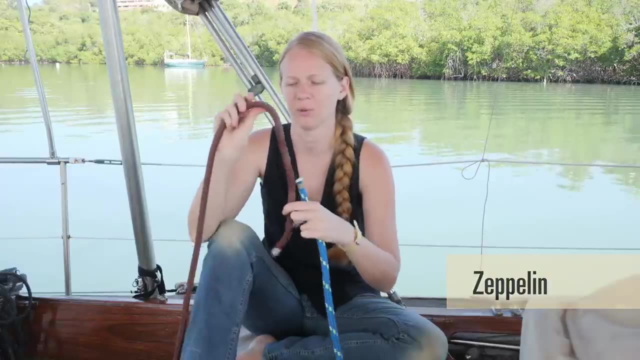 them together so that they don't come apart and so that, until you want them to come apart, that is okay. so the way that we do that is with something called a zeppelin knot, which might be a new one for some of you. the way we do that is: I create two fish in the line. see how I have a fish here and 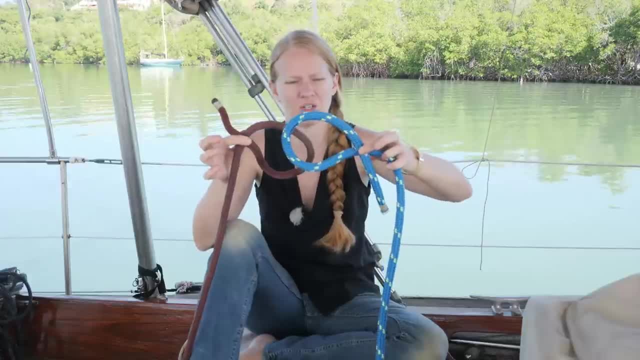 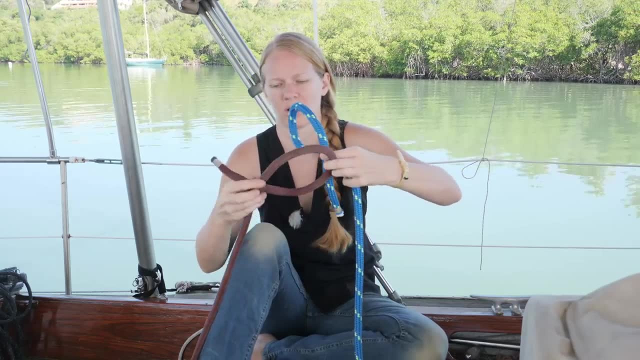 I'm going to have a fish over here. I'm going to make sure that you can see, here the tail. the shorter end is in front to you, and here I'm going to make sure that the shorter end is in back to you. I don't know how well you can see that. then I'm going to take the one that's in the back and 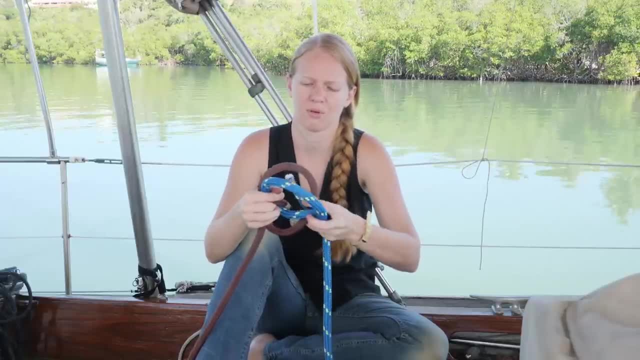 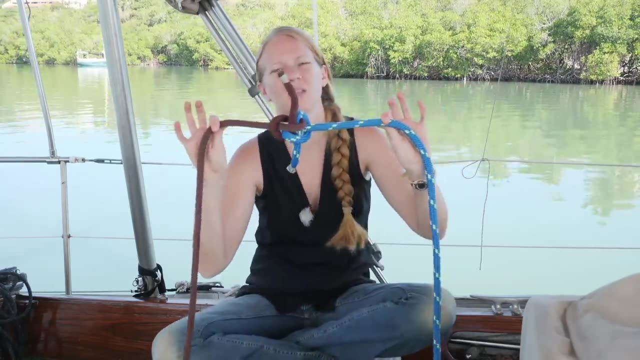 put it in the back and I'm going to make sure that the shorter end is in back to you so that back and the one in the front in the front, and trade them through each side and i get something that looks like this: this is a zeppelin knot and it's going to hold. 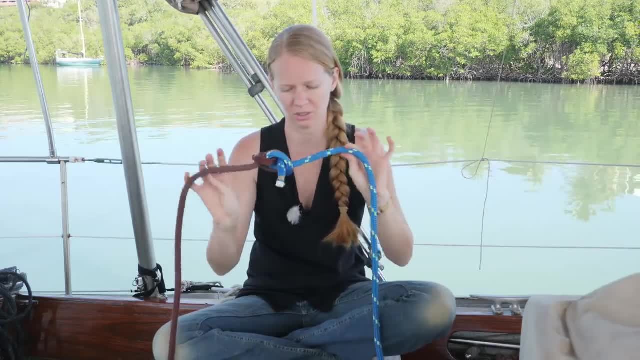 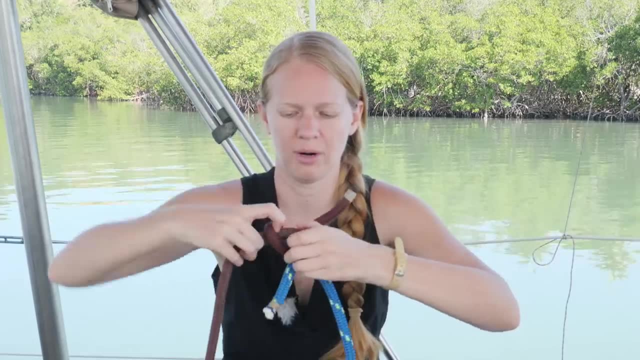 really tightly and keep these two pieces of rope together, remember. the other characteristic is we need to be able to get it apart again and you can see it's got this handy little loop, one on either side, so you just break its back. break its back and it comes right apart. 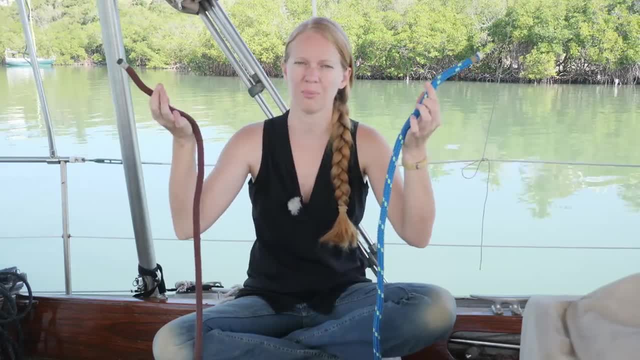 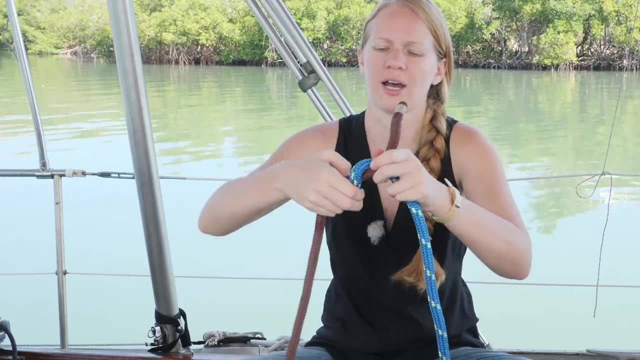 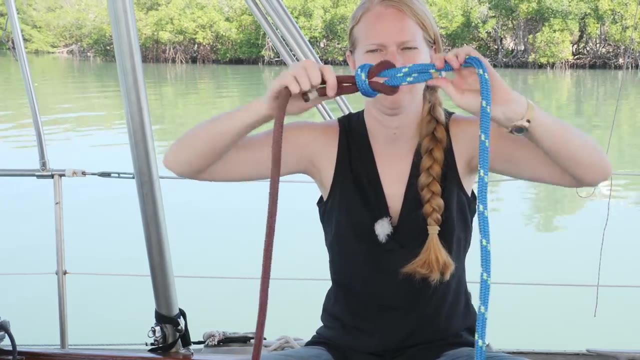 and that's a zeppelin knot. some of you might be saying, well, can i do a square knot for that? and you can, but there's a problem with it. let me show you so. if you tie a square knot there, we got a square knot right- what happens if, if anything, catches on this square knot you? 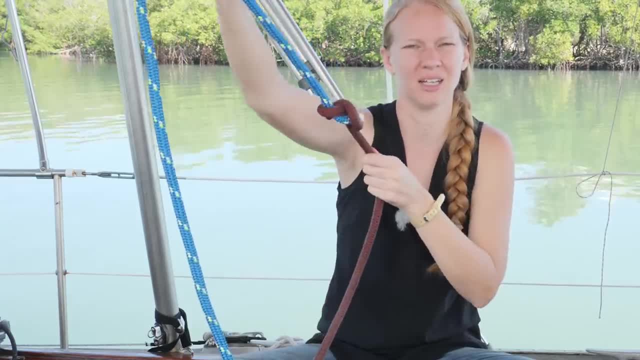 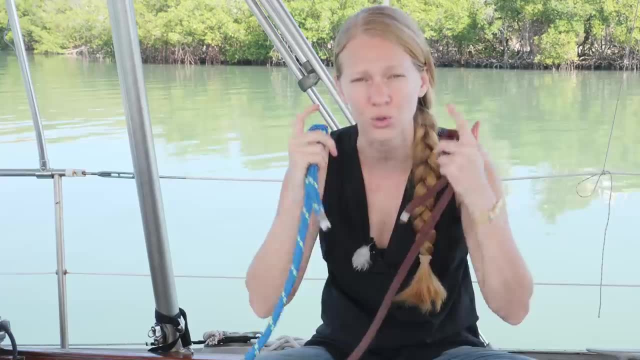 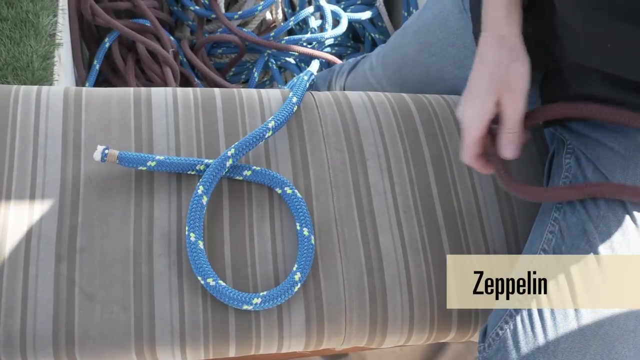 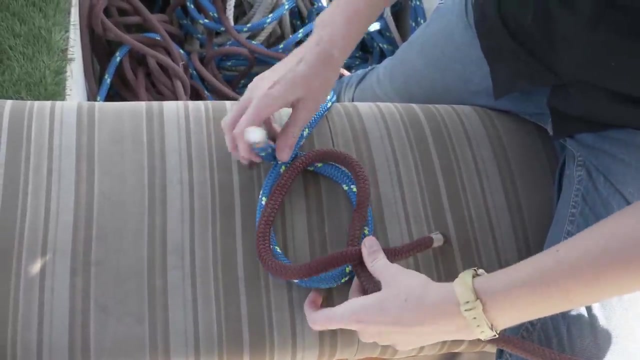 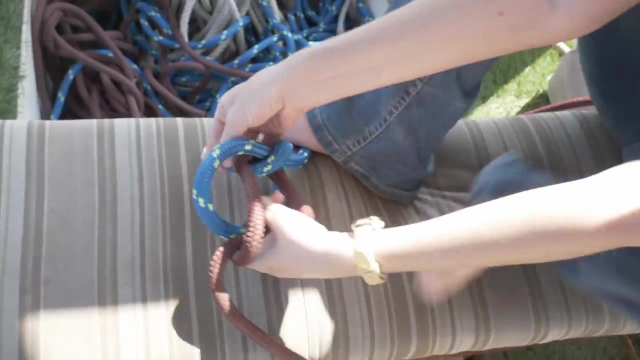 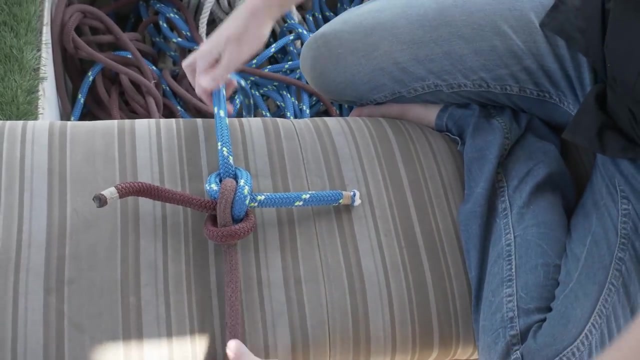 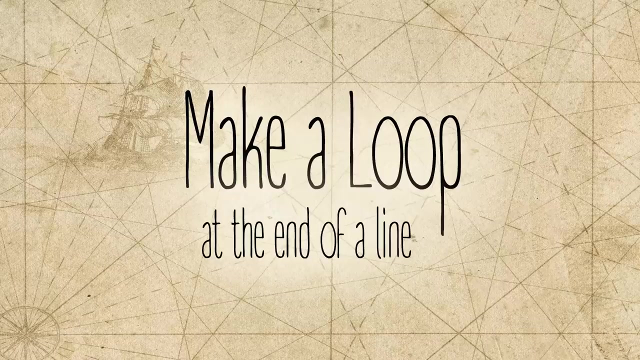 can easily transform it into something like this and something like this, which will pull right out. that's not what we want. so the zeppelin allows you something that's going to stay tight until you decide you want to pull it out. and the very last knot i'm going to show you is a bowline, which everybody knows. uh, if they're a. 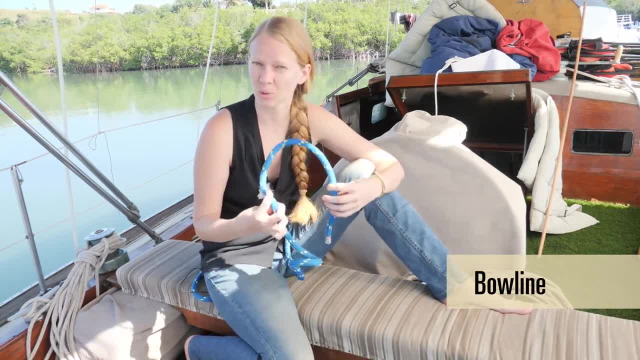 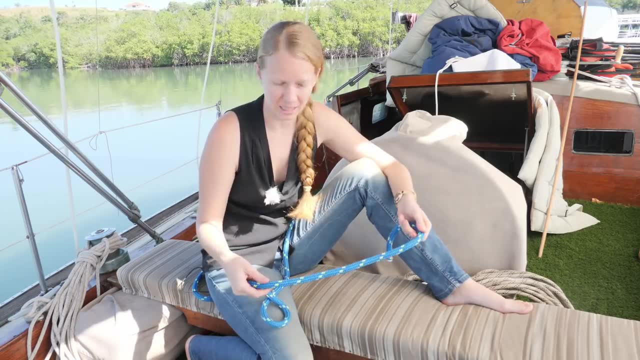 sailor, they all have a different way of tying it. i'm going to show you how i tie it and the shortcut way that clark sort of invented to tie it. both of them work pretty well, sometimes in different situations. the way i tie a bowline is to wrap it around. what i'm going to tie to 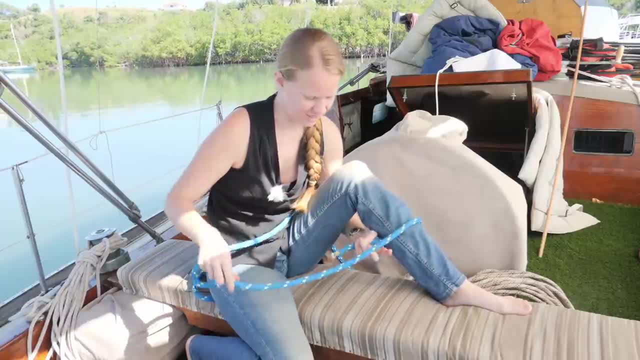 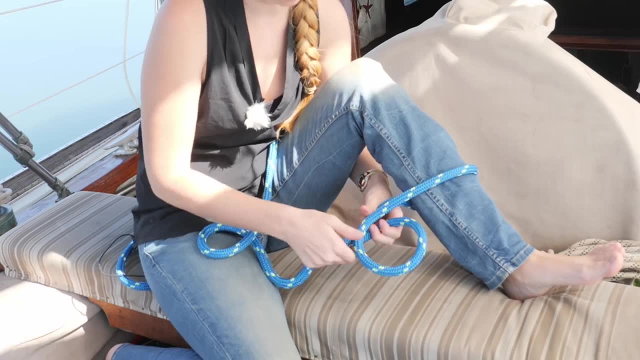 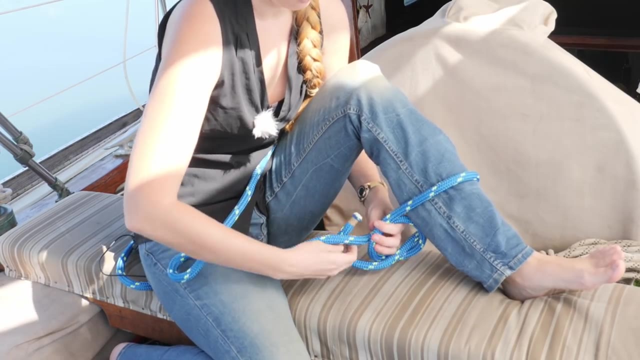 then i take the standing end- standing end, sorry- and i make a loop in it. i think of the standing end as the tree. so the tree grows from underground. i say a long tree grows from underground so you can see it coming up from underneath the loop. rabbit comes up and runs around back down the hole, out of sight, and 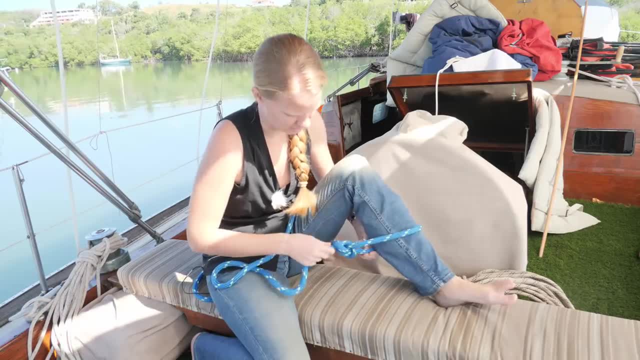 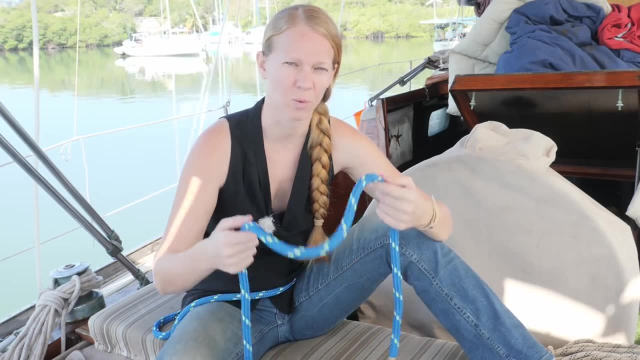 that's a bowline tied just right. so that's the way i tie a bowline. clark's way of tying a bowline is a little bit different, but it comes in handy when you have a little bit of prep time. but when it comes in you tie that bowline really quickly. so he does the prep work first, he does a little bit of. 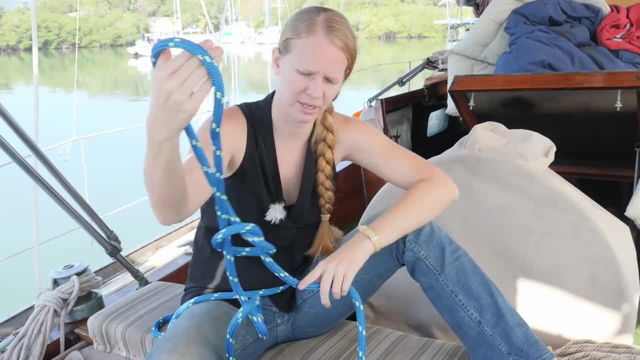 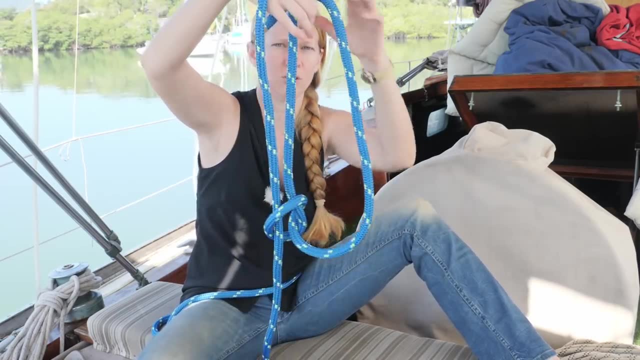 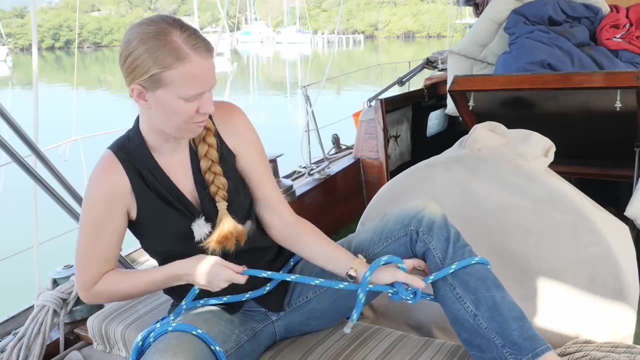 an overhand action here and passes the standing end loop through it and then all he has to do is put this through the loop and pull on the standing end. so the way this works, put it on my leg, pull this all the way through and pull that and kind of push it so it goes inside out. you'll 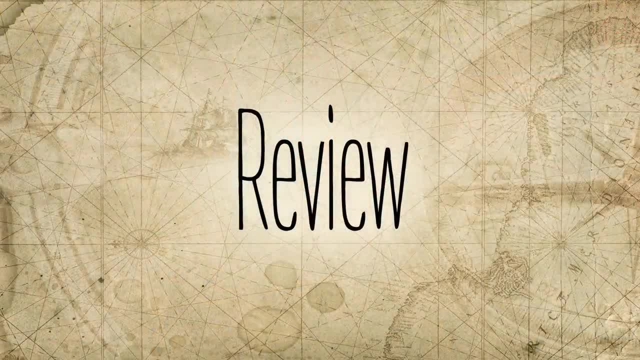 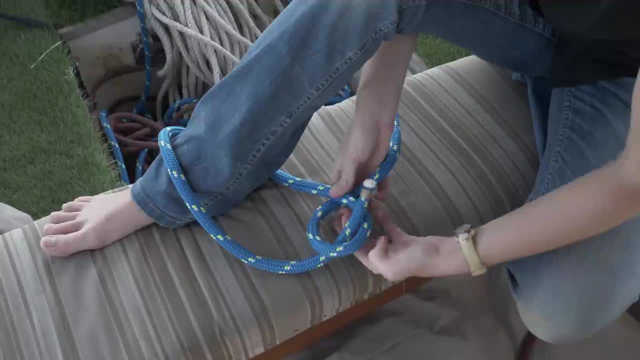 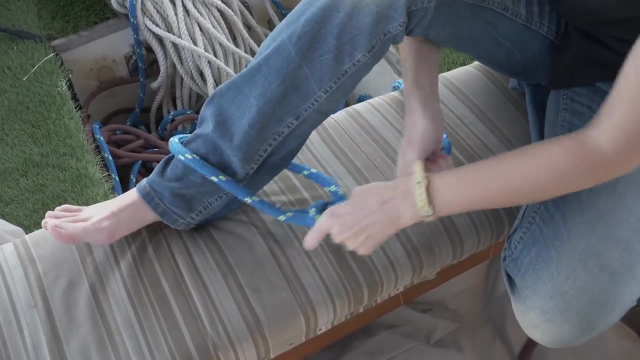 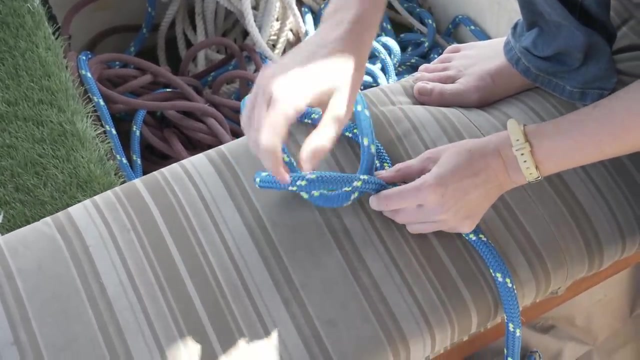 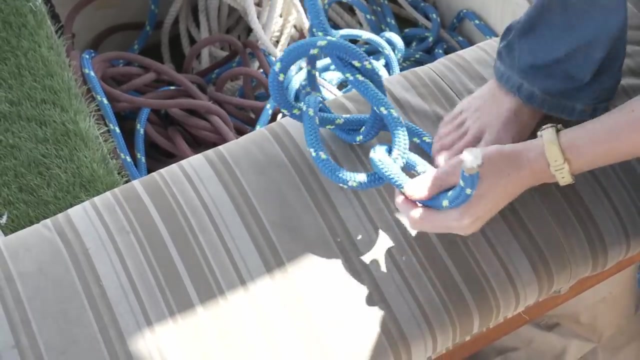 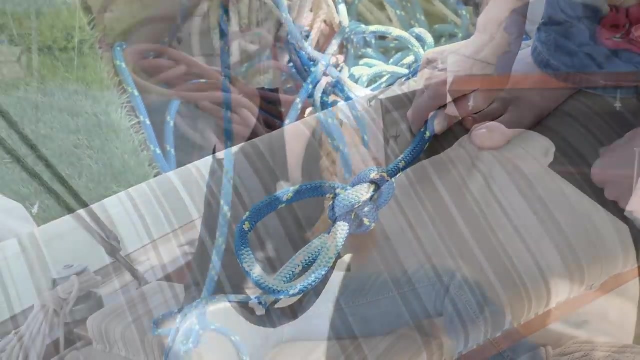 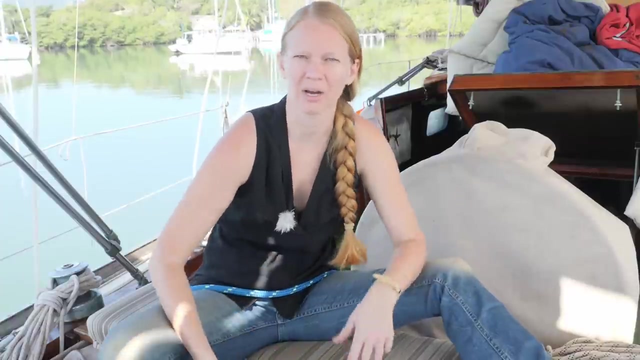 see that creates a bowline. do so, do so, so, so, so, So, if you can practice that and just practice all these knots, really, while you're sailing, while you're just sitting, keep a piece of rope in your pocket if you go to the waiting. 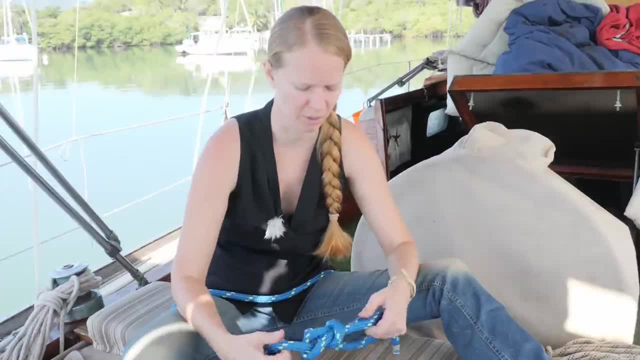 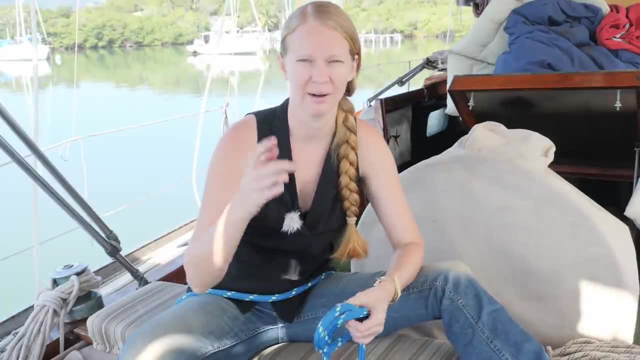 room or something. instead of getting out your cell phone, just practice some of these knots with a piece of rope And they'll get really good. they'll become sick in nature and make sure you know which ones to use when. Maybe we'll do that. I'll put up a little few slides at the end here and see if you. 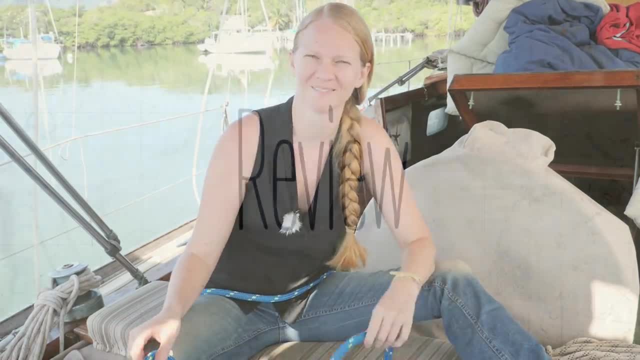 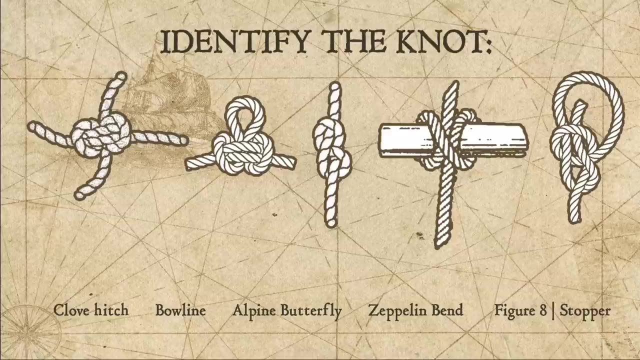 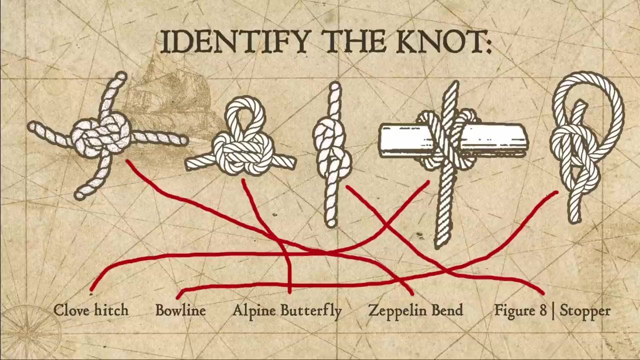 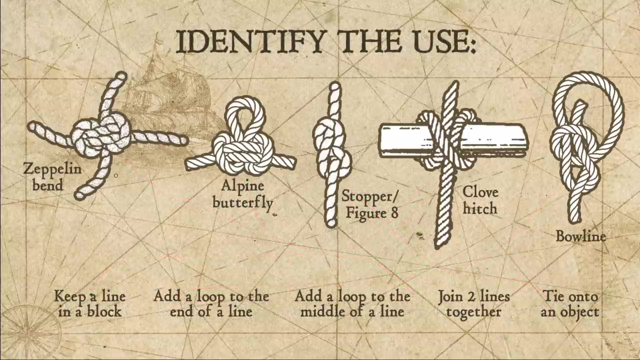 can match up the right knot with the right use, And then we'll come back and see how you do. And that's all the time we have for this video. Thank you for watching. We'll see you next time. Bye for now. 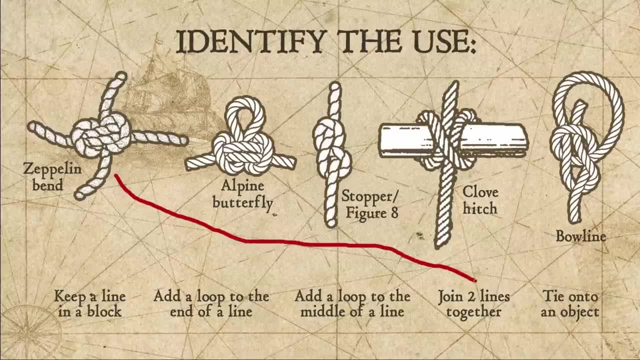 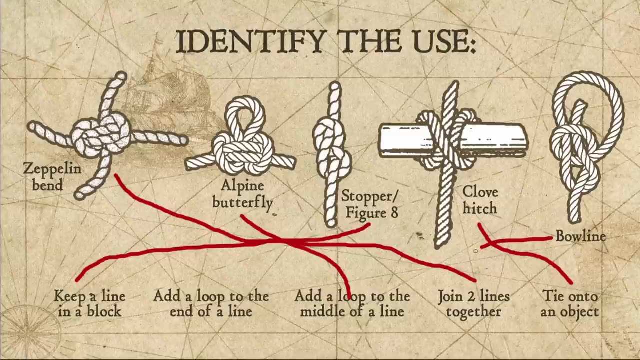 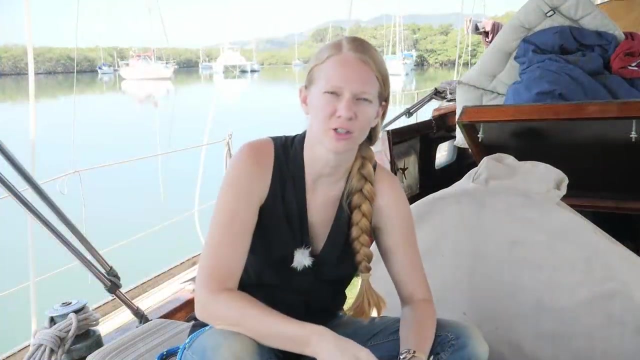 If you'd like to learn more about knots, there are two resources we can recommend. The first one is a book by Brian Toss called The Rigger's Apprentice. 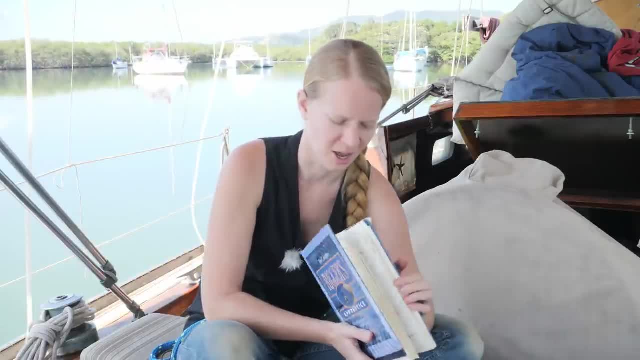 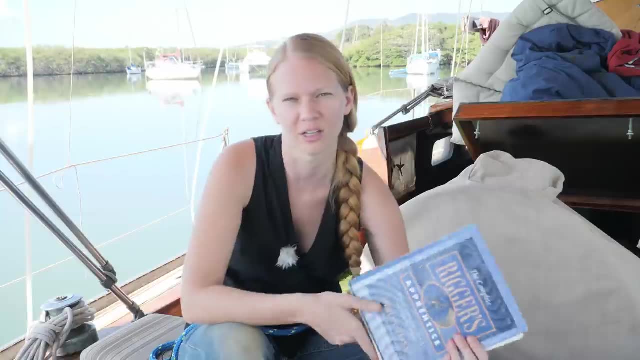 Ours is actually falling apart. We just got a new copy because we've used it so much. It's really well illustrated and walks you through step by step how to tie all kinds of different knots, even the decorative fancy ones that you don't need but are kind of 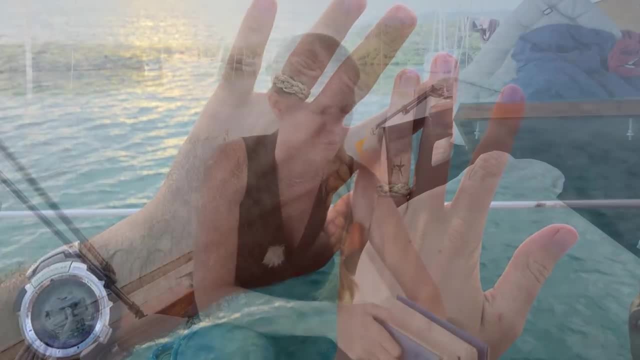 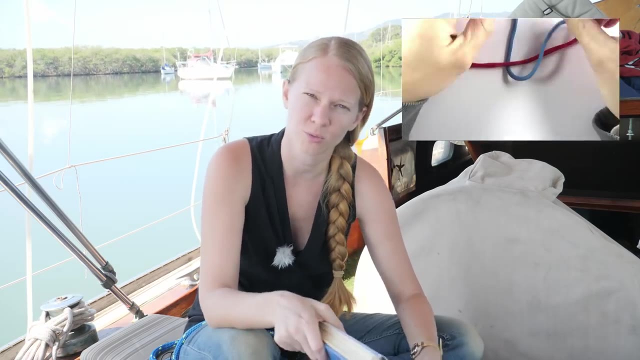 fun. We have wedding earrings that we made out of Turks heads and other fancy things that we've done on the boat. it's kind of a cool hobby to have. so check out riggers apprentice by brian toss. we'll put a link in the description and there's also a youtube channel called the paracord.